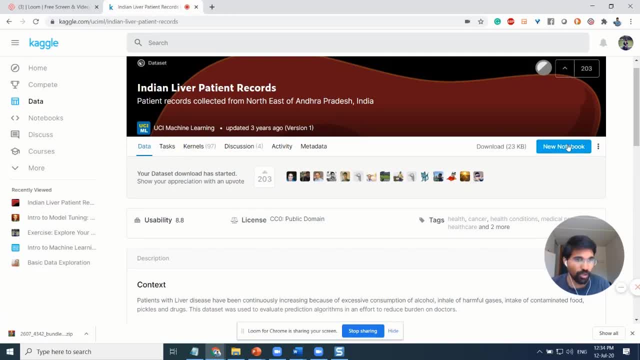 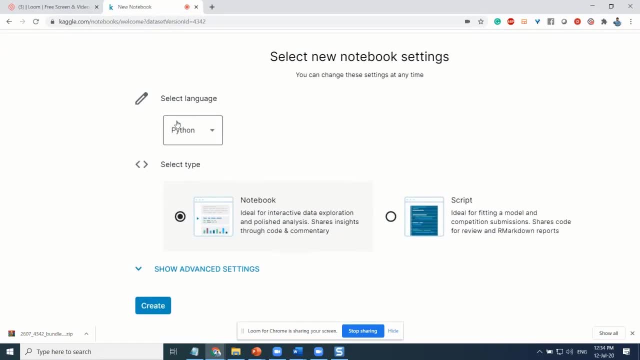 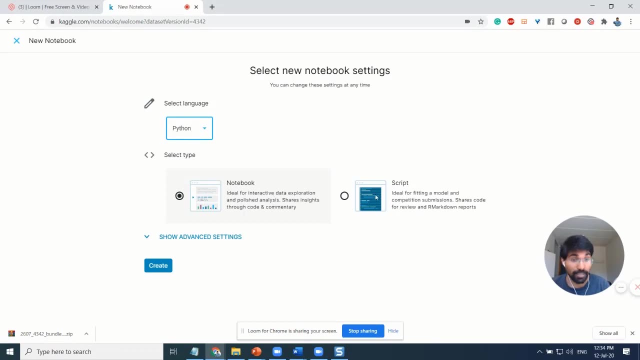 Kaggle for building your machine learning model. you just need to click on a new notebook that's available out here, So you just click on it. and then here you get to select your programming language. Here it can be Python or R, So I'll just go with Python. and also you can write a Python script. or you can create it in the form of a notebook, like a Jupyter notebook or a Collab notebook. Okay, so I'll just go with standard format where, like, I'm selecting Python and then notebook. Okay, I'll just create a notebook. 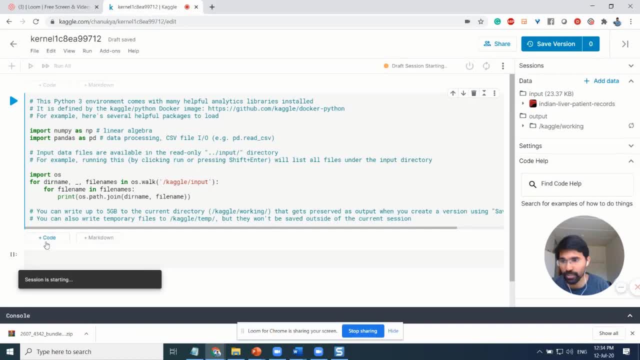 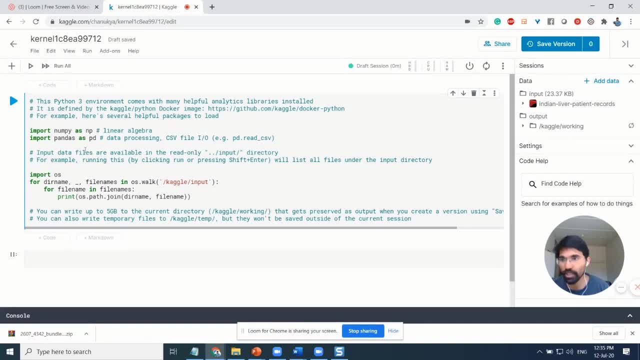 Here we already have some code that is by default given by Kaggle. It is nothing, but you are basically importing NumPy as NPA and Pandas as PD, And also you are importing the OS. Okay, so first thing that you need to do is you need to click on run so that you load your environment. 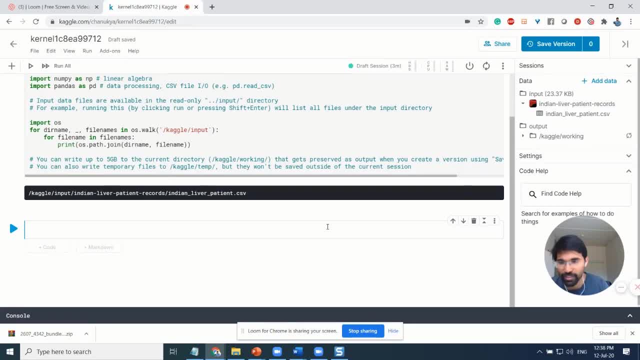 So we know how to read a CSV file, right? So let's create a variable called as data, an object called as data, And let's read it as a pbread underscore: CSV. And if you don't remember, it's fine. 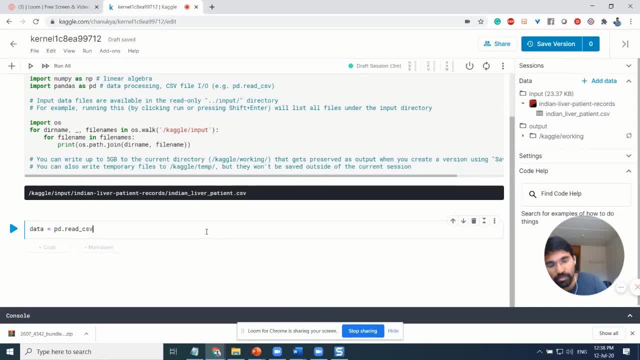 And then we can search it on. I'm really sorry, I'm using a Dutch keyboard. So yeah, you just need to copy paste your file path in this particular space. So how do you do it? So, basically, you have your data set here. 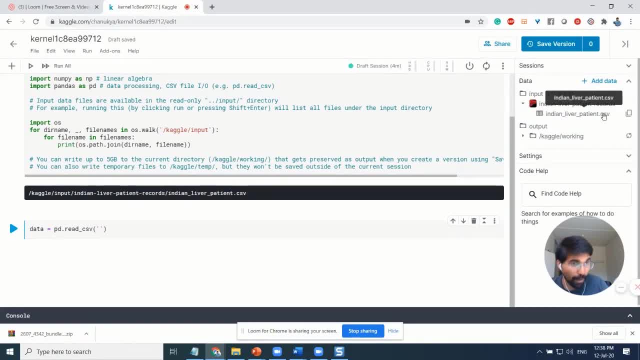 You just need to click on this and then you will find the path to the CSV. So you just need to click on copy file path and then paste it here, Then run the code. Okay, after this is done, you can also check the head of this particular data set. 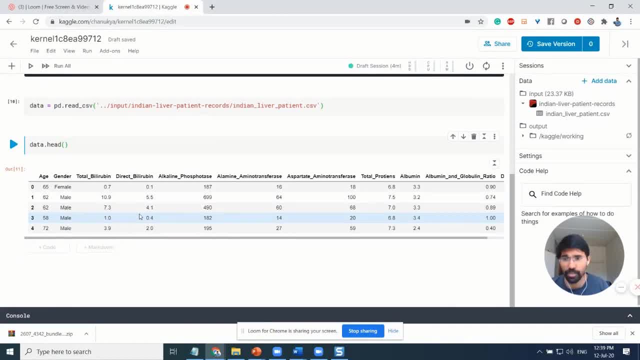 You can read the entire data. Okay, and from here on, you anyway know how to do the exploratory data analysis, And you would know how to do a bunch of other things. right, You can do your data preprocessing. You can build your own machine learning models after that. Have fun and good luck. Take care, Bye, Bye, Bye, Bye, Bye. 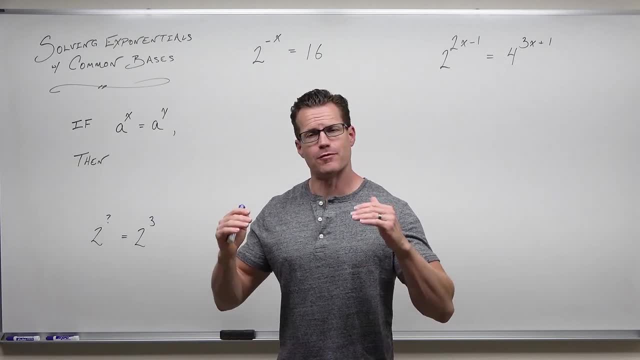 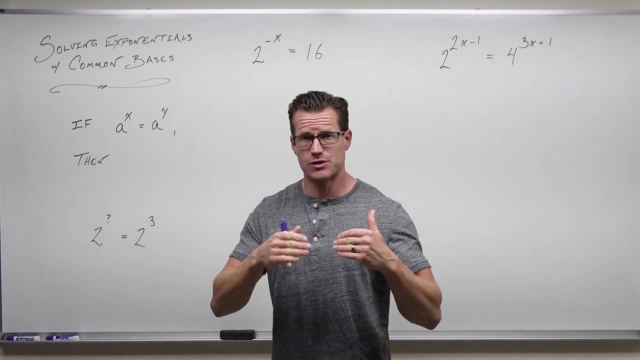 Hey, welcome to another video. So in this video we're going to talk about a very special case on how to solve exponentials. So we are kind of halfway through talking about exponentials and logarithms. We're going to get to logarithms very shortly, but we're going to talk about 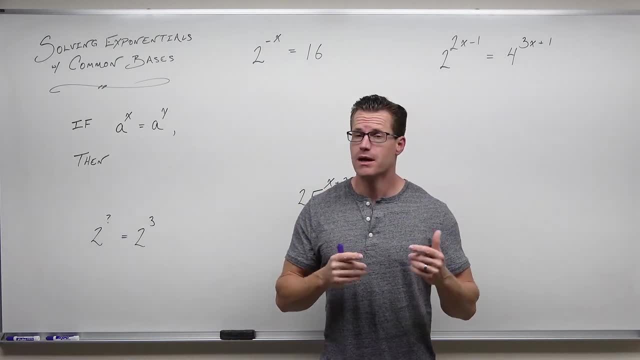 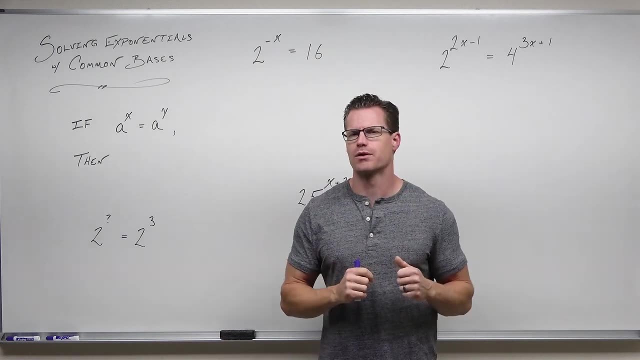 exponentials, just to get our brains wrapped around, a couple of ideas. So here's what I want you to learn in this video. Number one in general, why we have learned everything we've learned in this unit. so talking about exponentials and logarithms and inverses and one-to-one functions. 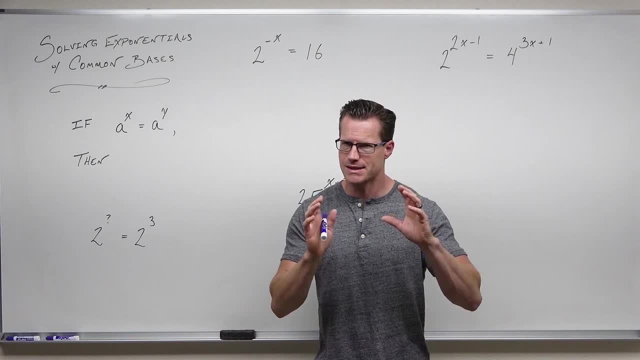 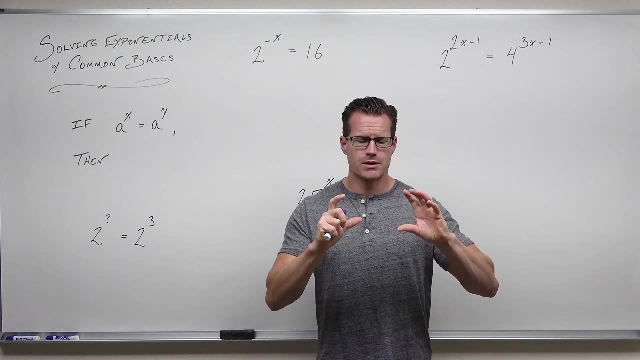 and composition functions is so that we can make the following connections: This is it. This is the train of thought that we needed to know. Number one: we learned about one-to-one functions so that we could discover inverses. One-to-one functions have inverses. We learn about inverses. 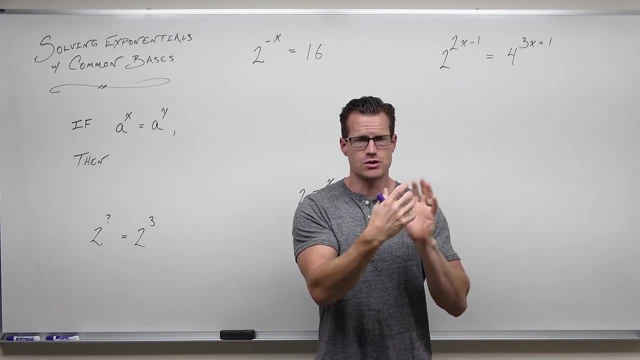 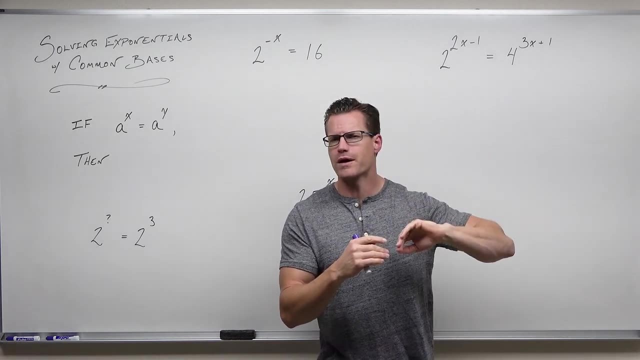 to know that when you compose two inverses of compositions with inverses, they undo each other. We learned about those things to discover that exponential functions are one-to-one, Therefore they're going to have this inverse. We're going to call that inverse a. 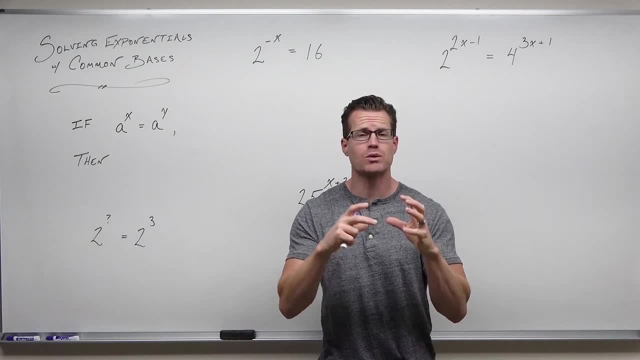 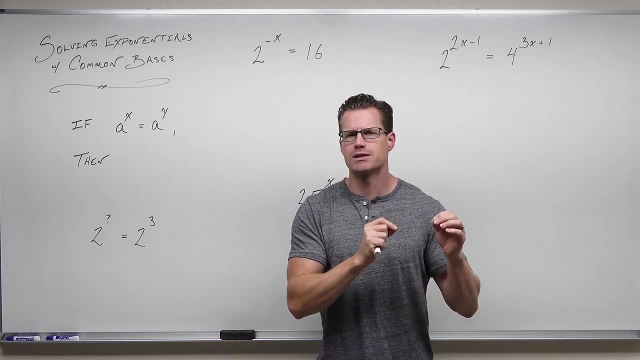 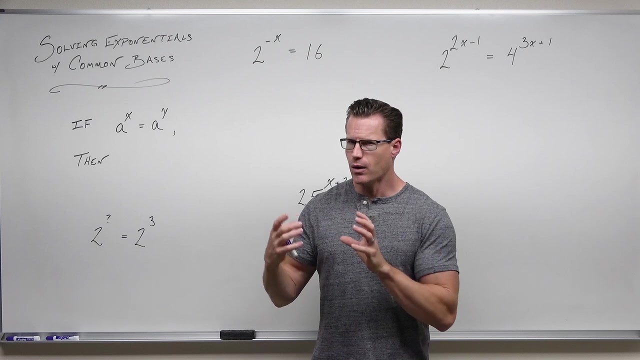 logarithm and when you compose them, an exponential and a logarithm will basically cancel each other out. That's what we're going to get to. So this is a very, very special case on what if you can shortcut that situation, What if you can solve exponentials without logarithms? And there is